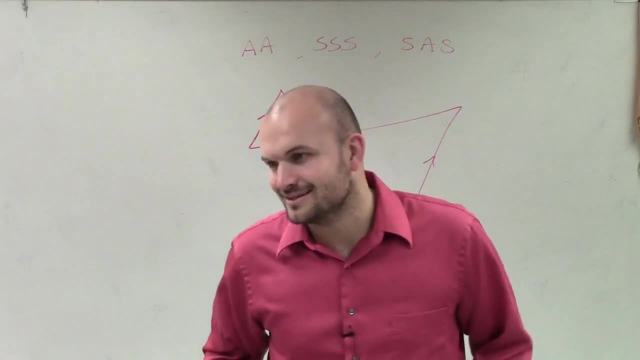 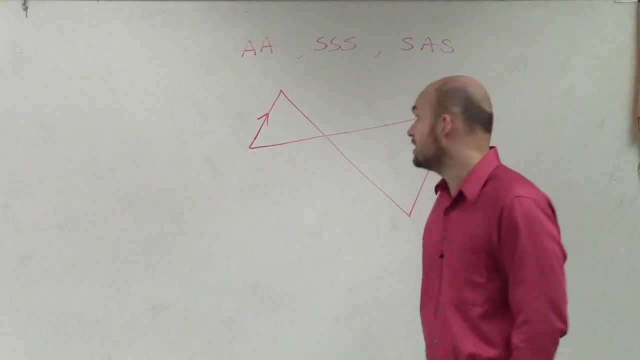 I know I was trying to think of what to say and I whatever What. In my home country, that's the way that we'd say it. OK, So let's go and talk about some things. So, Kevin, if it's similar, why are they similar? 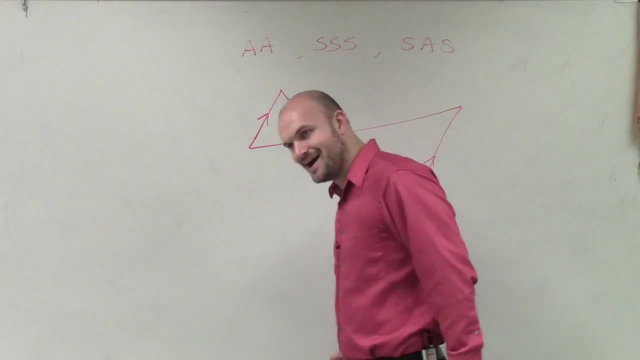 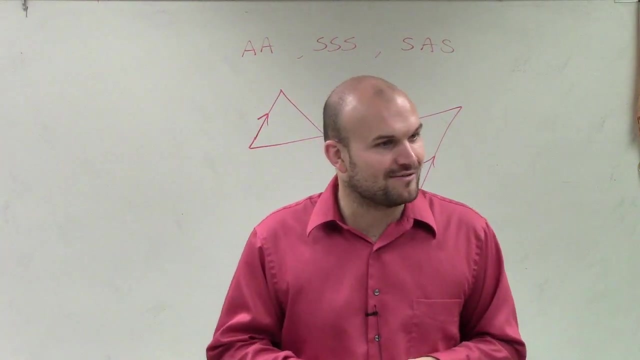 Whoa, whoa, whoa. Kevin, slow down. You're just knocking this out of the park, All right. so for some people that are not as amazing as Kevin for seeing this, let's go and identify what he did. 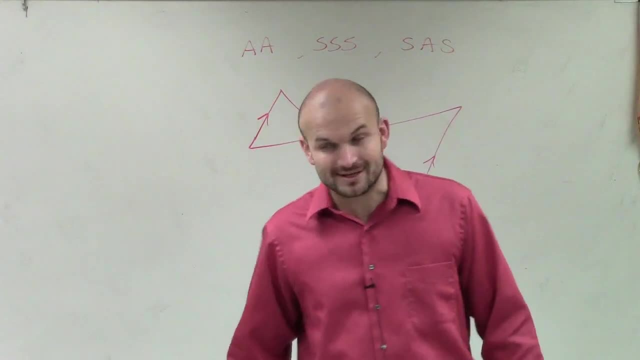 because he hit it nail on the head Last class period. it was like a 10-minute video I had to help them out with so awesome job. So the first thing, guys remember. there's a couple different options we look at. 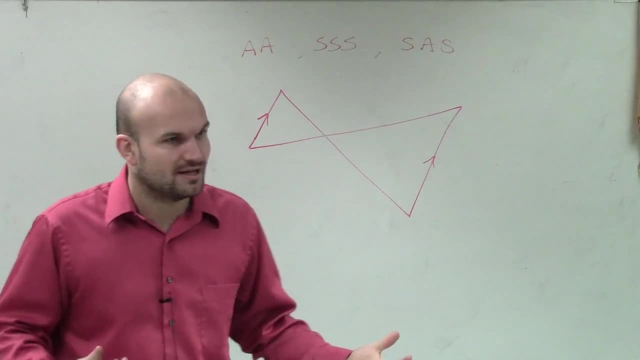 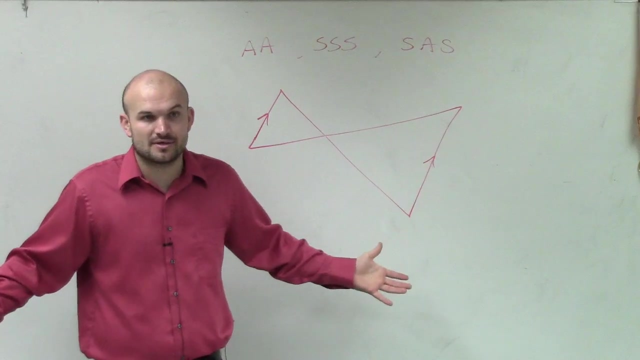 First of all, what you guys want to do is look at this problem and see what is it you are given. The only thing you are given is these parallel lines. That's it. That's the only thing they tell you about this. So to say that the length is equal. 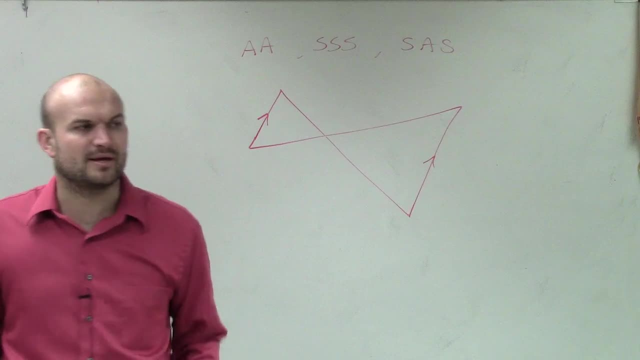 the lengths are going to be equal. it's going to be very, very difficult to do. Just put it in the side bin, right? So therefore, that would make me think of all right, I have to go and prove that angles are congruent. 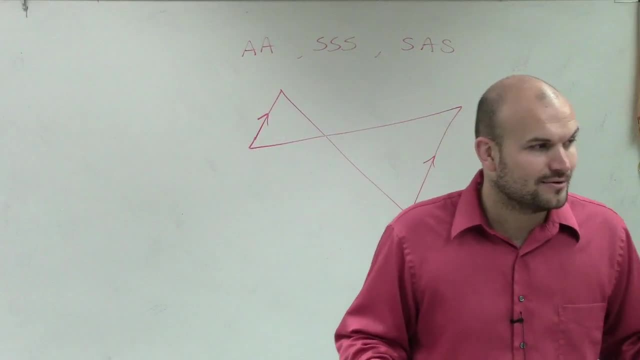 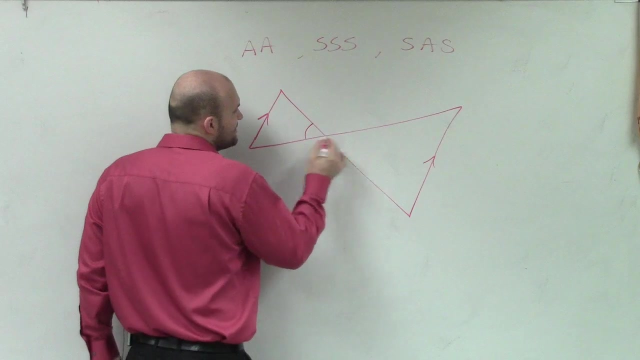 Now we know that when we have parallel lines, then we have parallel lines and a transversal, we have angle relationships. But I'll get to that in a second. The most obvious one, I would say, would be these two angles right here. 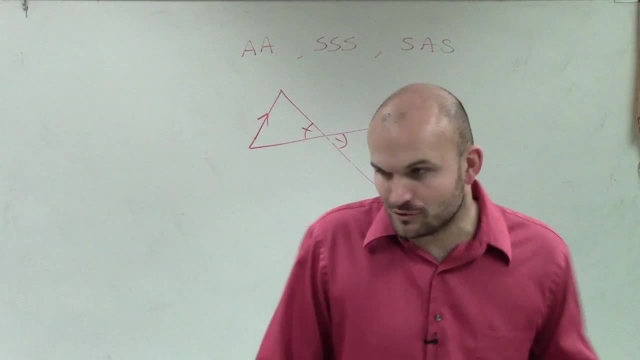 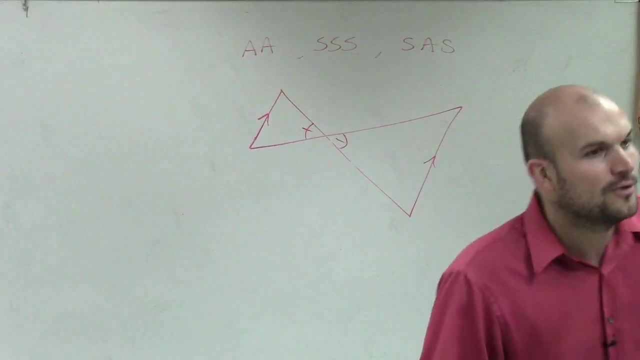 Because, hopefully, since the beginning of the year, I have drilled into you that when you have intersecting sides that do not share a side but share a vertex, we call them vertical angles, And vertical angles are equal in measurement right, So we can say that these two angles are congruent. 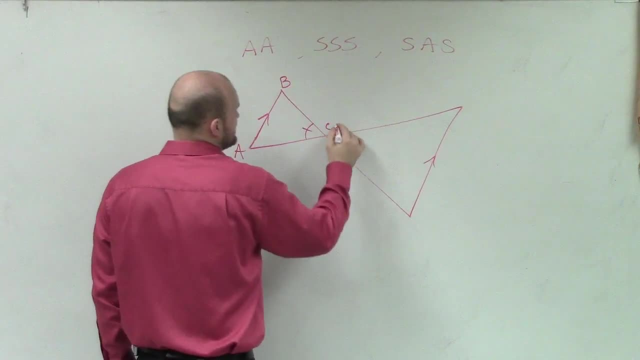 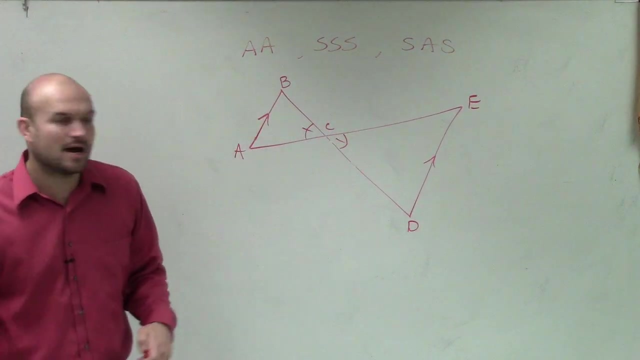 Oh, let me write this down. So I'd say A, B, C And let's call this D, E, D, D. OK, So we know those are equal. Now, where Kevin did a great job, is he understood? 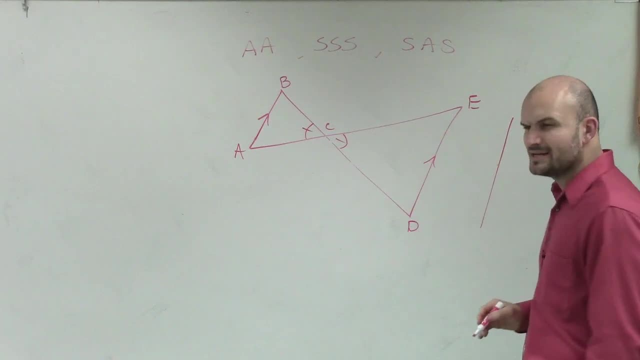 that these lines are parallel, And what angles did you say were equal to each other, Kevin? Which ones? The vertex is both of them, B and D. OK, so let's call them A, B, C and E D C. 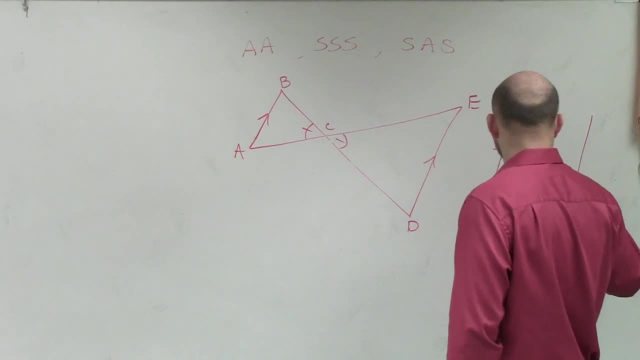 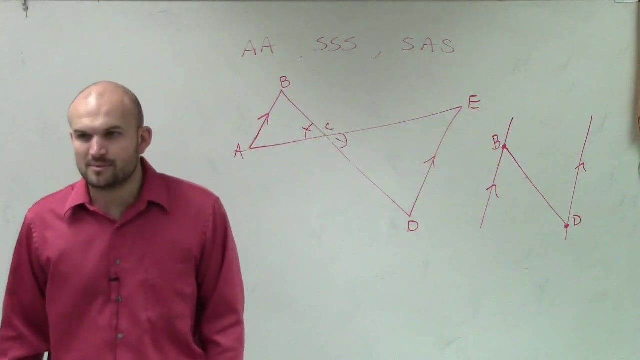 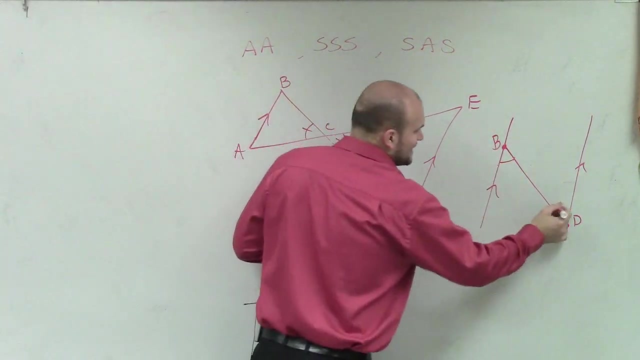 So he's saying that let's pretend we have B and we have D. And if I was to draw a straight line to them? so these lines are parallel. Does everybody remember problems like this? You have a set of parallel lines. He's trying to tell me that this angle is equal to that angle. 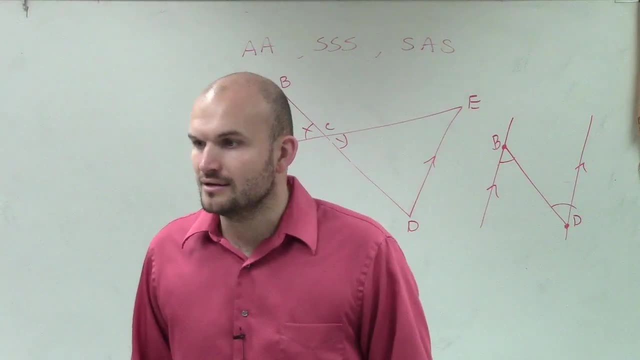 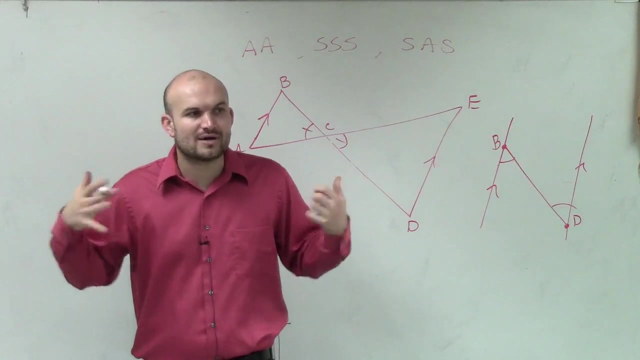 If those lines are parallel and you have a line that intersects, are those two angles equal to each other? Yes, So, ladies and gentlemen, when you're looking at a problem like this, try to look past, just looking at triangles. Try to see what information can I. 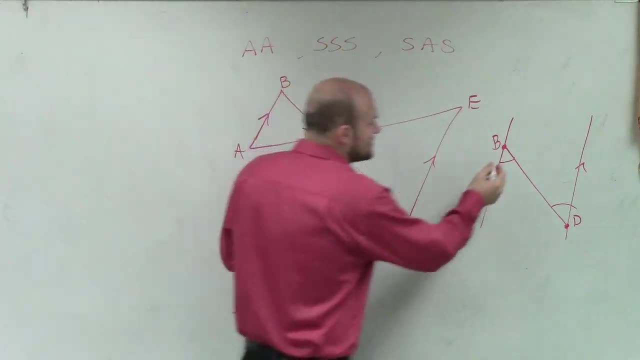 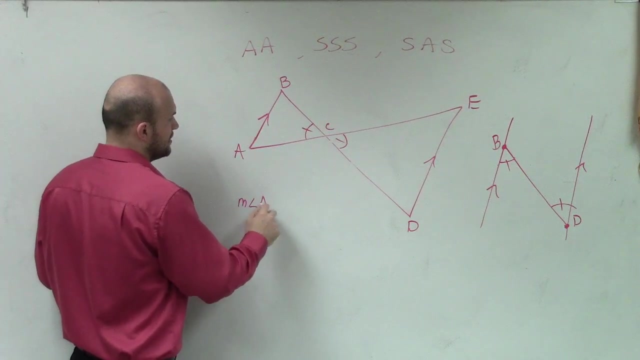 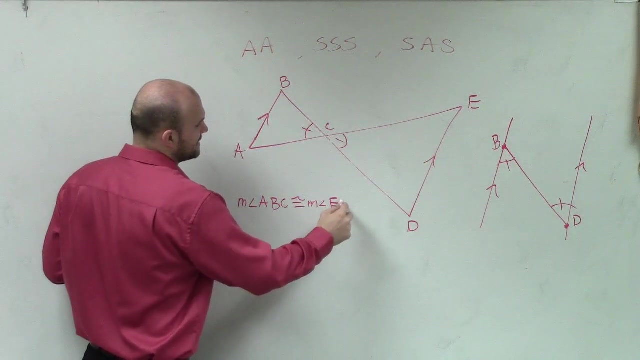 take from this to determine Because, yes, he's absolutely correct, Those are equal to each other. So what I can say is measure of angle A, B, C, D, E, D, C, B, C is congruent to the measure of angle E, D, C. 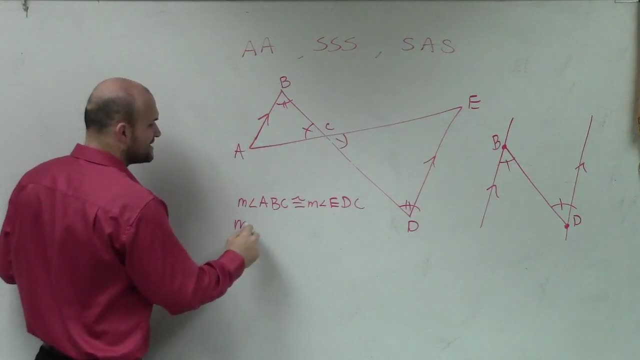 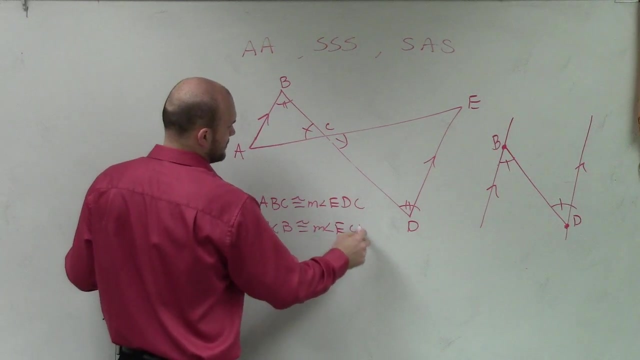 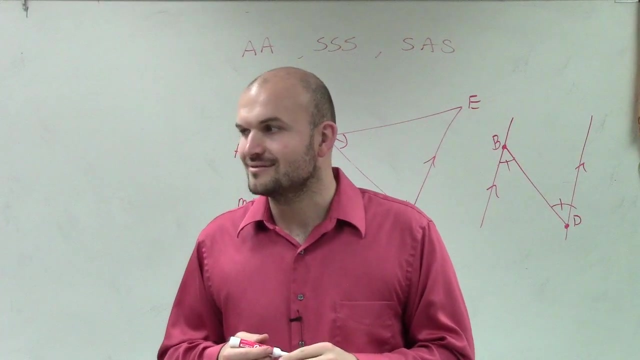 which is right here and right there. Then I can say: the measure of angle A, C, B is congruent to the measure of angle E, C, D, And since we have two angles that are now congruent, can we now say these are similar? 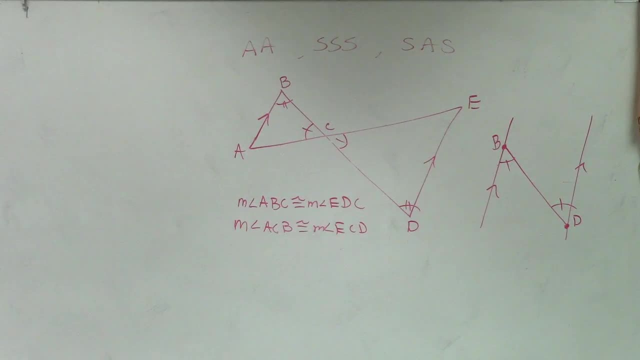 Yeah, So we're good Cool.